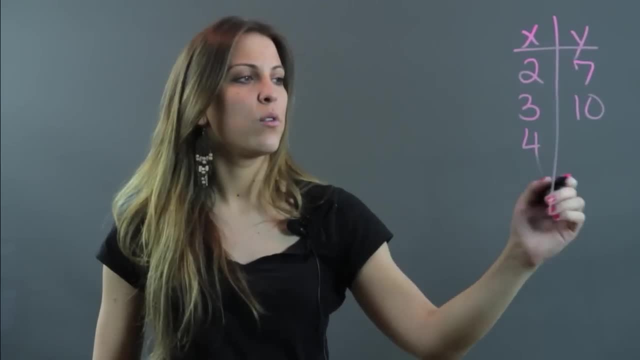 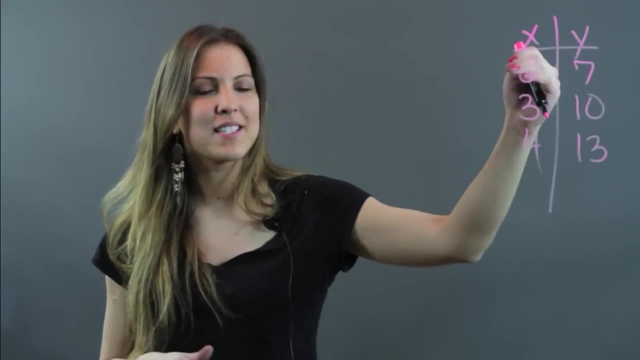 is 3, and my y is 10, and my x is 4, and my y is 13.. Alright, so what you're doing is looking to see if there is a relationship between x and y that's consistent with all of your ordered pairs. So there has to be something that I can do to this x, For example. 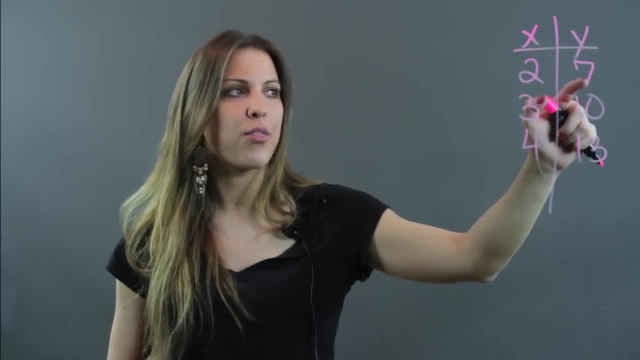 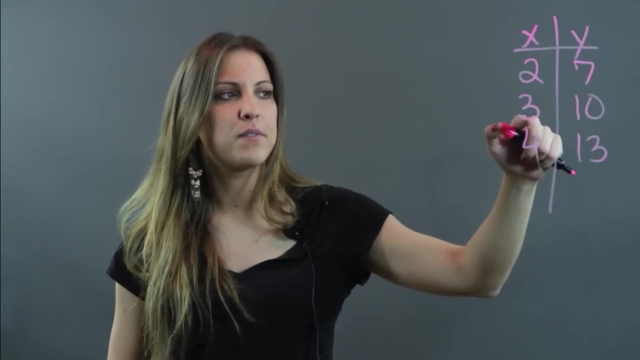 I can multiply that x by 5 and then subtract 3 from it and I'll get that y right. 2 times 5 is 10, minus 3 is 7.. But if I try to do that here, 3 times 5 is 15, minus 3 is not. 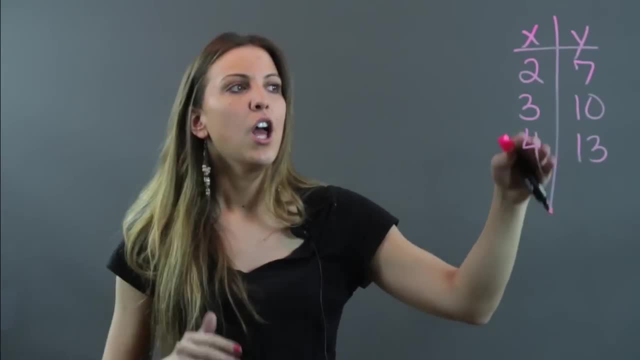 10.. So that's not the relationship I'm looking for. I'm looking for something consistent. You can sort of guess your way through it until you find it. I think the easier way to do it is to first find the slope of the equation. 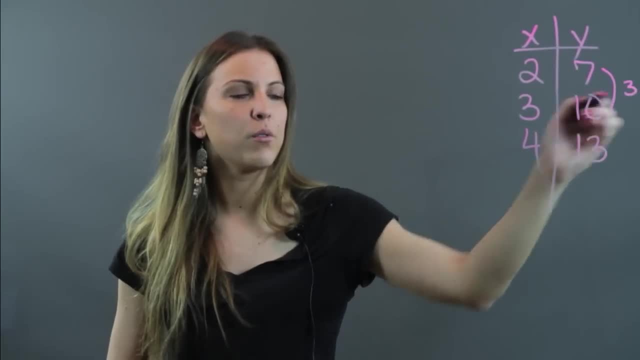 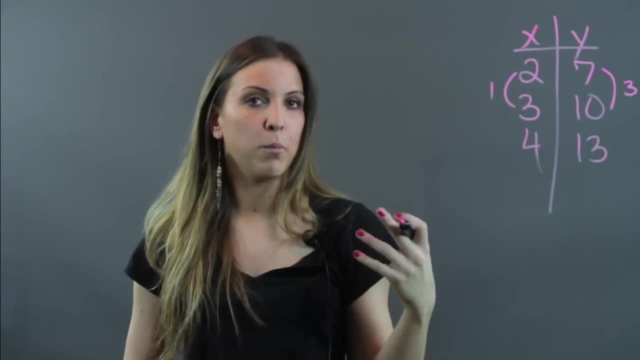 So I ask myself: how do I get from 7 to 10?? Well, I have to go three spaces. And how do I get from 2 to 3? I have to go just one space. So my y over my x becomes my slope of whatever. 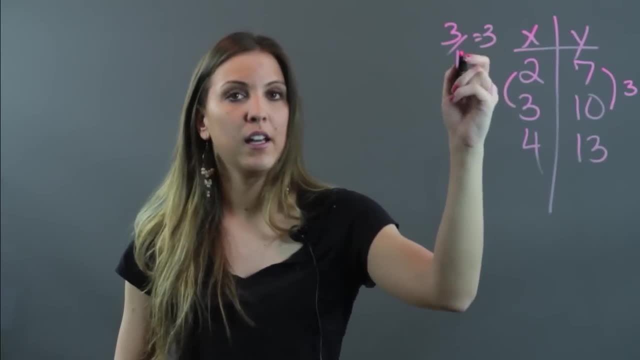 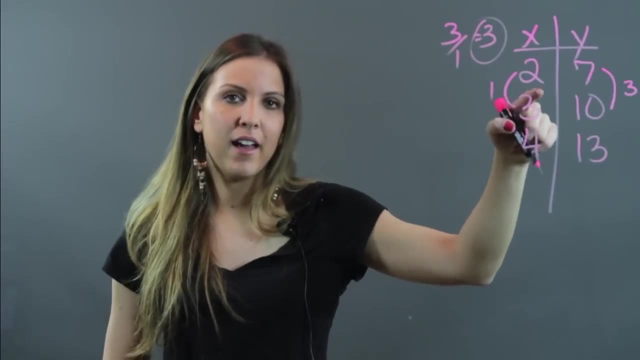 line I'm creating. So 3 over 1, or just 3, is my slope. This is important because that means that's the number that I'm multiplying x by. So if I know that from there, it's a little easy to see what I have to add or subtract to it to get to the rest of the y. So 3 times. 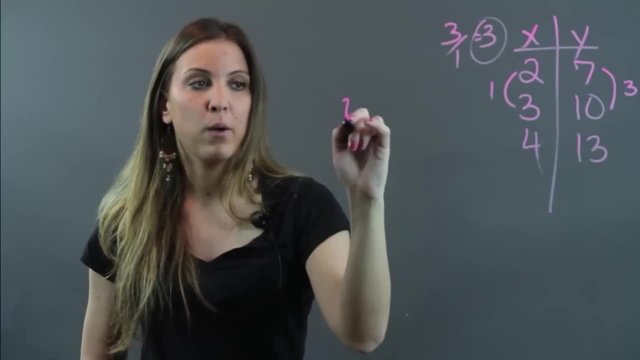 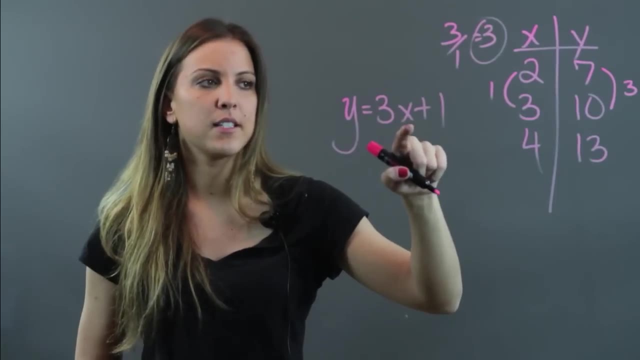 2 is 6, and to get from 6 to 7 I have to add 1.. So my equation would be: y equals 3x plus 1, if it works for all the others. So let's see: If I take 3, 3 times 3 is 9, plus 1 is 10.. That is my y value, And 4, 4 times 3 is: 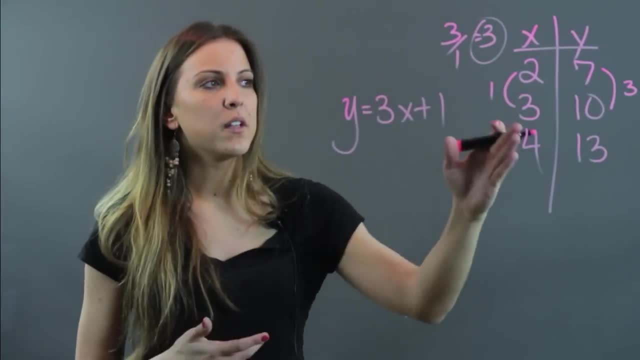 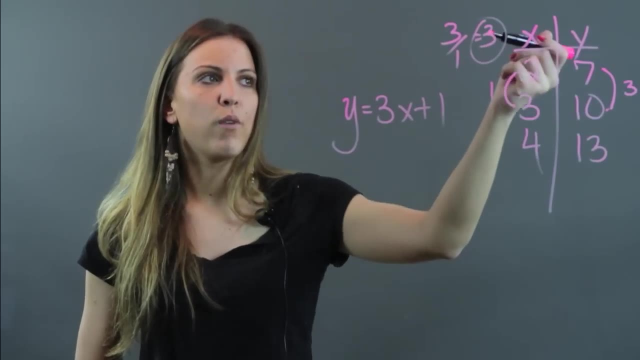 12, plus 1 is 13.. That is my y value as well. So you can sort of guess and check. I think the easier way to do it is find the relationship between your first two y values, your first two x values. write it as a fraction. That's the number you're going to multiply x by. 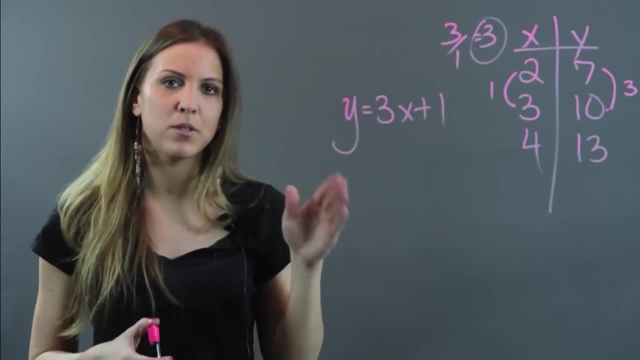 My name is Maria and I just showed you how to figure out whether there is a linear relationship between a table of values And how to write their equation.